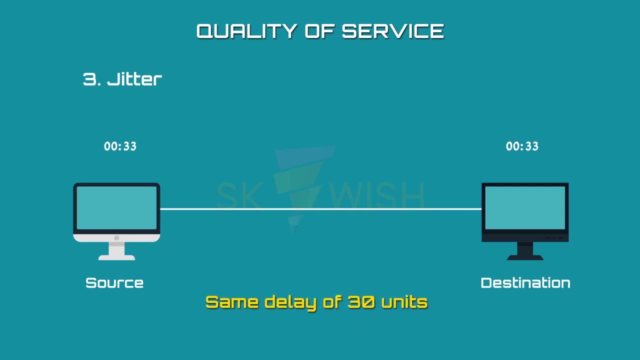 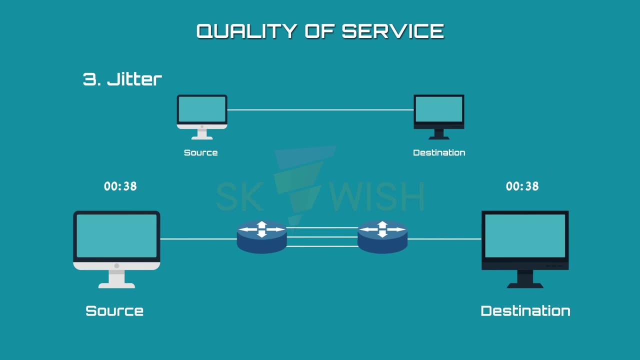 32,, 33, all have the same delay of 30 units. On the other hand, if the above packets arrive at 33,, 31, and 38, they have the same delay of 30 units- they will have different delays For audio and video transmission. the first case is completely. 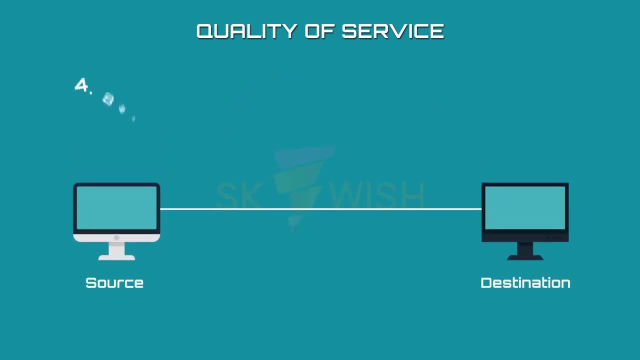 acceptable. The second case is not Bandwidth. A network needs appropriate bandwidth for a specific application. For example, video conferencing needs to send millions of bits per second. This needs higher bandwidth, While file transfer may not reach even a million bits. 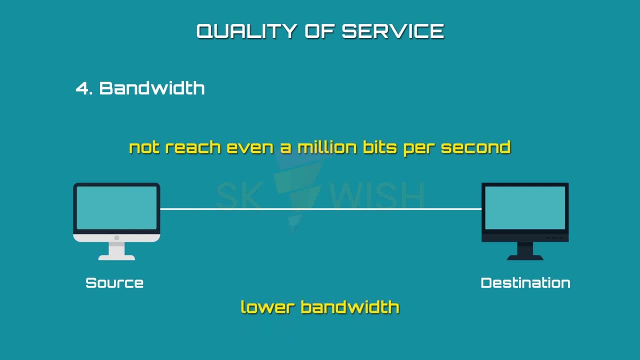 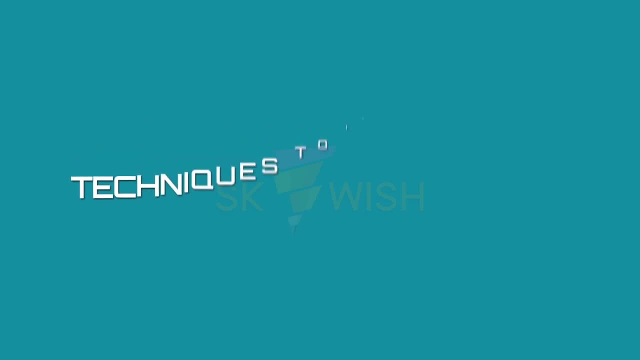 per second. a lower bandwidth for this application is acceptable. Now we will see the techniques to improve quality of service, Techniques to improve QoS. We must improve the quality of service of a network for reliable delivery of data. There are some techniques to improve the quality of service. 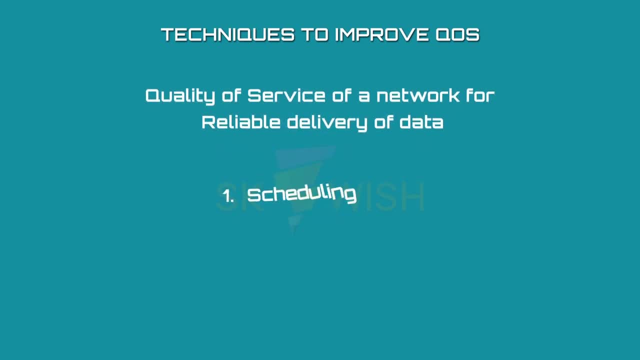 We discuss some of them. They are scheduling, traffic shaping, admission control and resource reservation. Scheduling: Usually a router or a switch gets packets from different flows for processing. All the packets from different flows must be treated fairly to get a good quality of service. 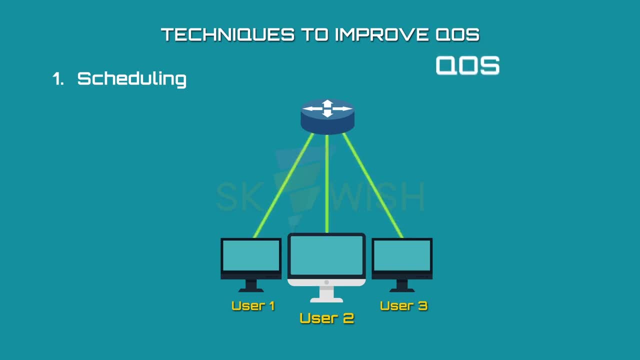 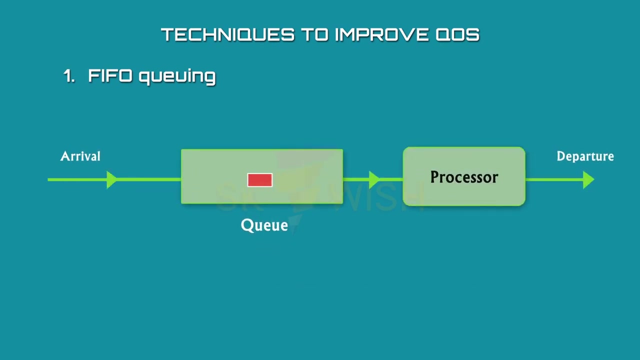 We discuss some of the scheduling techniques that improve QoS. They are FIFO queuing, priority queuing and weighted fare queuing. FIFO queuing: This is called first-in, first-out queuing. In this method, packets wait in a buffer or queue until the node is ready to process them. 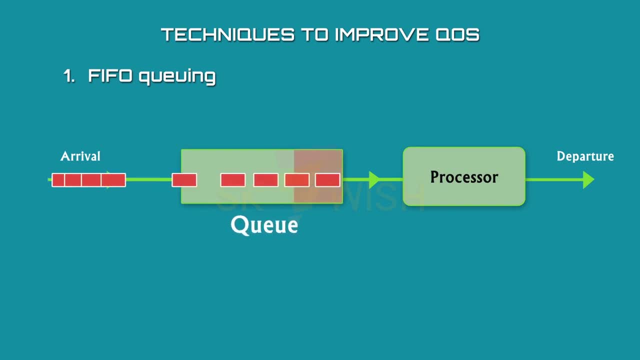 If the arrival rate is higher than the processing rate, the queue will fill up and the new packets after that will be discarded. Here the oldest entry is processed first, That is, the packets leave the queue in the order in which they arrive. 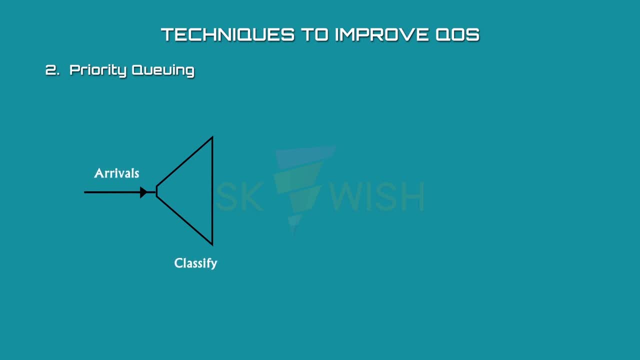 Priority queuing. Here we have two types of queues: Higher priority queue and lower priority queue. The packets as they enter are first assigned to a priority class. That is, time-sensitive data goes to higher priority queue. Other data, like file transfers, goes to lower priority.